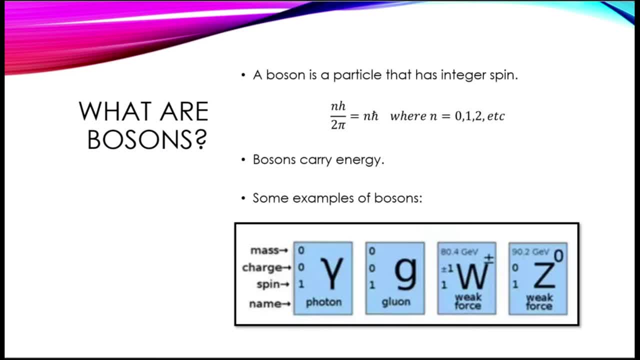 what are bosons? A boson is a particle that has integer spin. The spin of the particle can be written as n, which is just an integer. In this case, h is Planck's constant and divided by 2 pi. When h is divided by 2 pi, we can abbreviate it as h bar. Bosons are particles that carry energy. 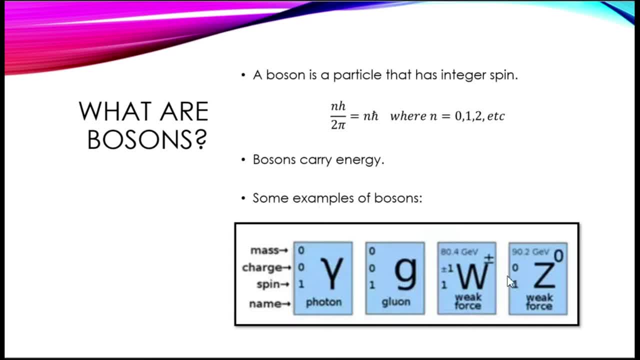 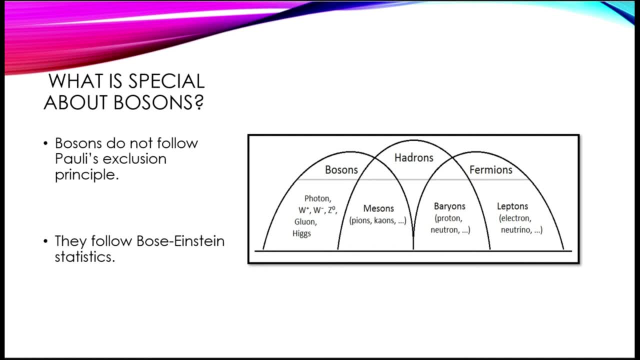 and some examples of bosons are the photon, the gluon, the w and z bosons. So what exactly is special about bosons? Well, bosons do not follow Pauli's exclusion principle. Recall that Pauli's exclusion principle states that two or more identical fermions 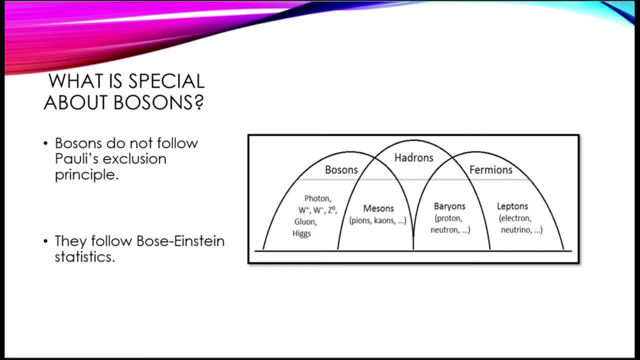 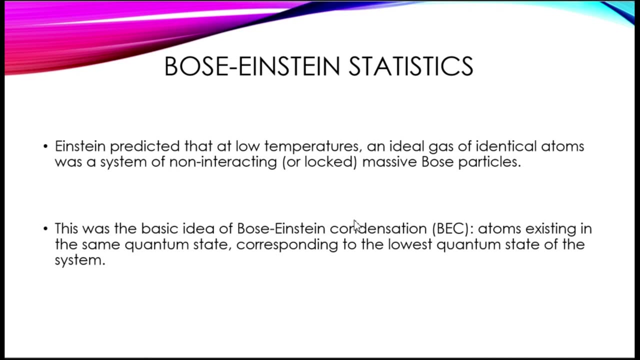 which are neutrinos, leptons, quarks, electrons, cannot occupy the same state. Instead, bosons follow what is called Bose-Einstein statistics. So how was Bose-Einstein condensation discovered? Well, photon statistics, which is the quantum statistical property of a. 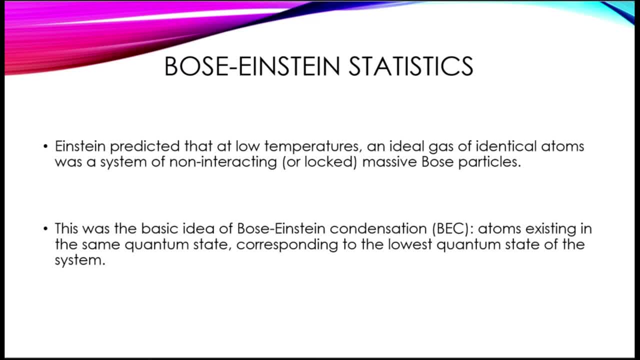 massless Bose particle was first studied in 1924 by Bose. This work was later generalized by Einstein to an ideal gas of identical atoms. He predicted that at low temperatures this ideal gas was a system of non-interacting or locked massive Bose particles. This was the 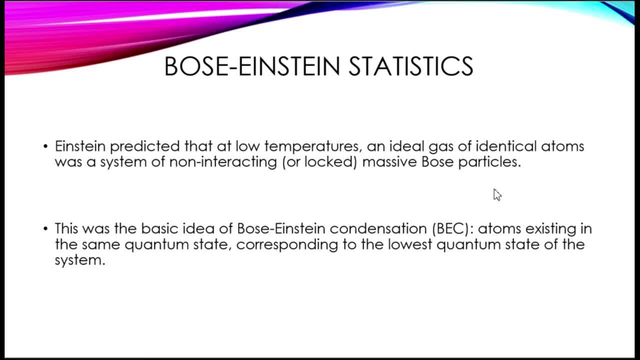 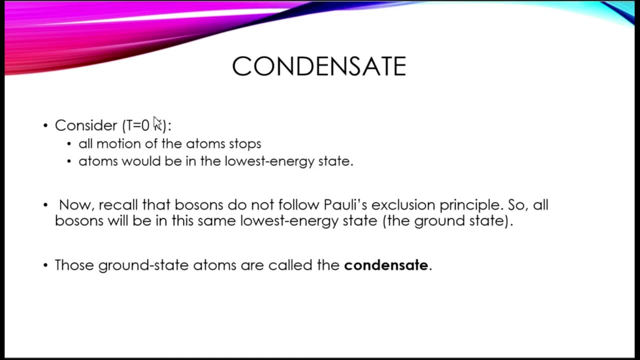 basic idea of Bose-Einstein: condensation: atoms existing in the same quantum state, which corresponded at the lowest or grand state of the system. So these atoms are called a condensate. So considering the temperature of absolute zero, at this temperature all motion of the atoms stops And the atoms would be at lowest energy state. 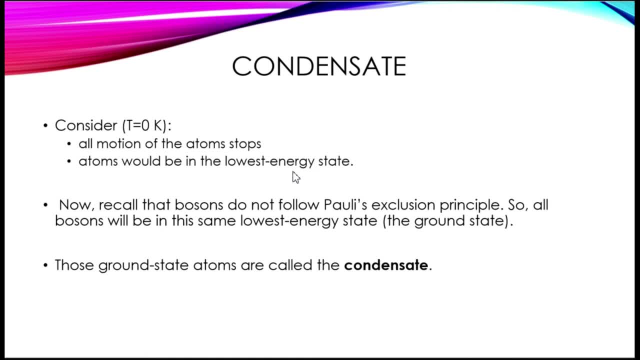 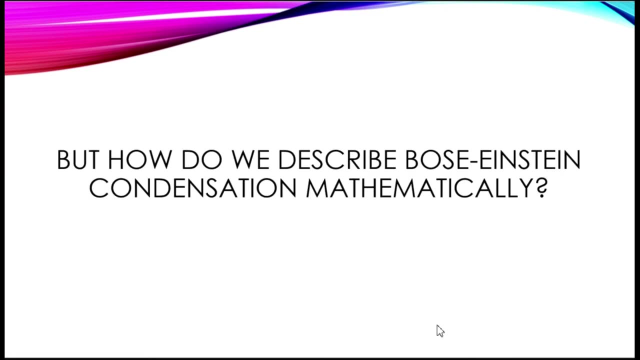 Now recalling that bosons do not follow the Pauli's exclusion principle. all the bosons would then be able to be able to stay in the lowest energy state, energy state at the same time, so the ground state. So how do we describe Bose-Einstein? 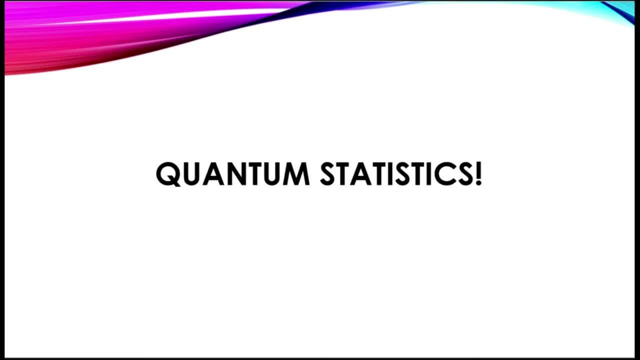 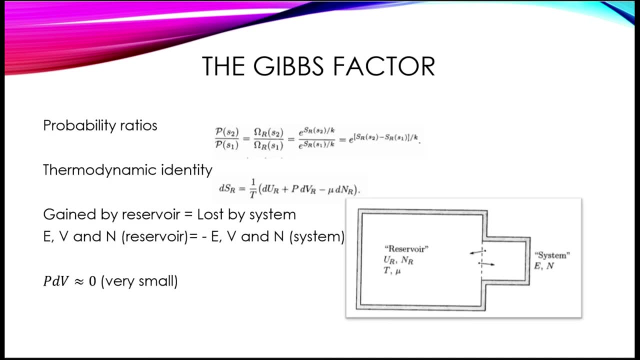 condensation mathematically. Well, for this we use quantum statistics. So before we can describe Bose-Einstein condensation, I need to explain a few concepts of quantum statistics. So I will start with the Gibbs factor. So this derivation is very similar to the derivation of 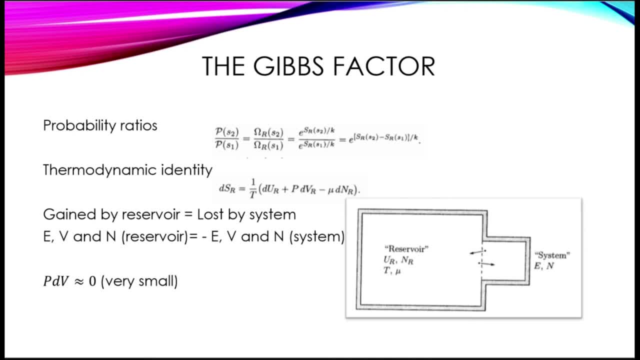 the Boltzmann factor for an isolated system where all the accessible microstates are equally probable. And the isolated system here is the atom and the reservoir together. So we write the probability ratios of an atom being in state 2 versus state 1, just like we did in chapter 6.. 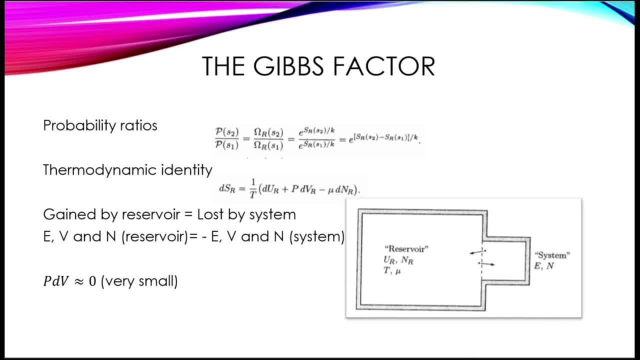 Recall that the probability is multiplicity over number of microstates. So then we can express the probability ratios as shown in the table, And then we can notice here that the exponent has changed in entropy, which we can then use the thermodynamic identity to further explain. So remember that whatever is gained by the reservoir, 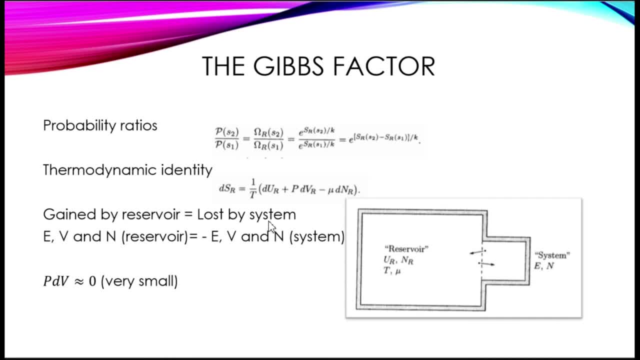 must be lost by the system. So in this case, if we have the energy volume and number of particles of the reservoir, that should be equal to the number of particles of the reservoir. So in this case we can set Pdv as approximately 0, because it's typically very small compared to the other numbers. 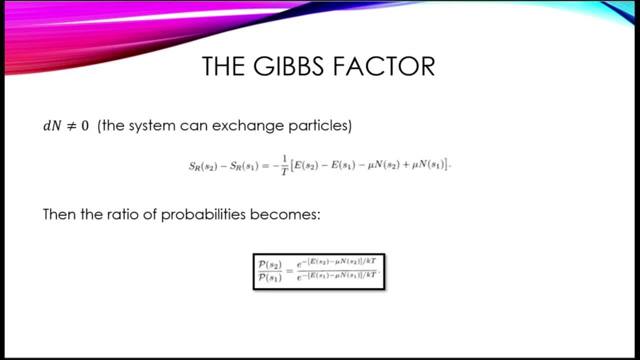 Now remember that when we derived the Boltzmann factor in chapter 6, we used the thermodynamic identity too, But we assumed that no particle transfer occurred and set dn to 0. In this case we will assume that the system can exchange particles, So dn is not 0. 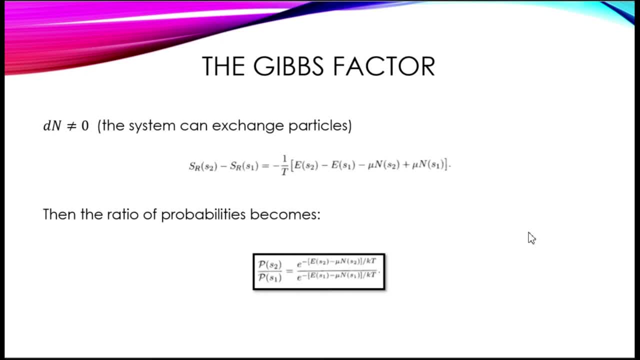 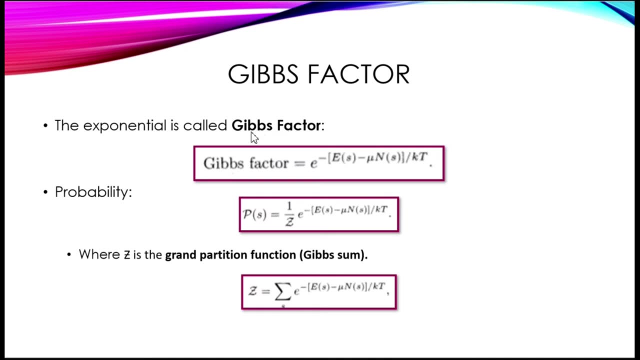 So then we can express the difference in entropies as shown here, And the ratio of probabilities becomes this expression. So here you notice there's an exponential part, and that exponential part is called the Gibbs factor. So if we want absolute probability, we need to divide it by a constant of proportionality. 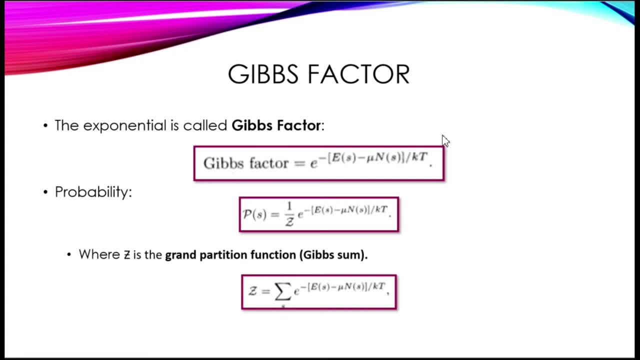 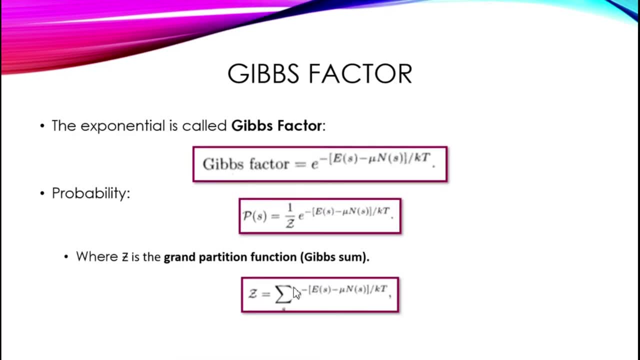 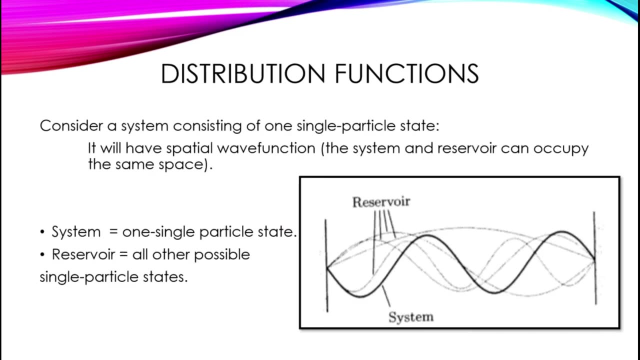 that would make the addition of probabilities equal to 1.. So that constant is called the grand partition function and is used to give terms. So something else we need to understand is the distribution functions. So if we consider a system consisting of only one single particle state, 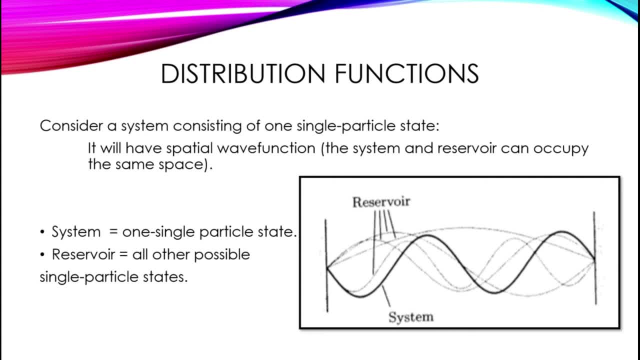 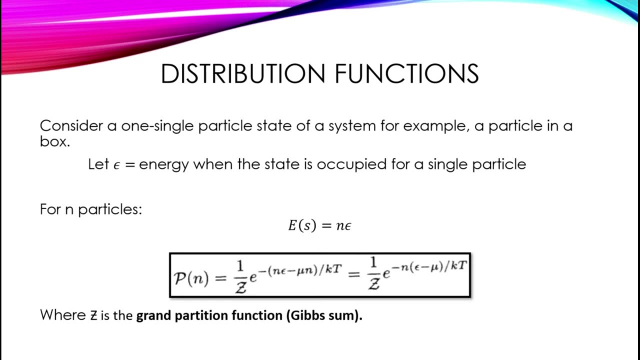 it will have some spatial wave function And in this case the system and the reservoir can occupy the same space because we're talking about bosons. So the system here is a one single particle state and the reservoir is all other possible single particle states. 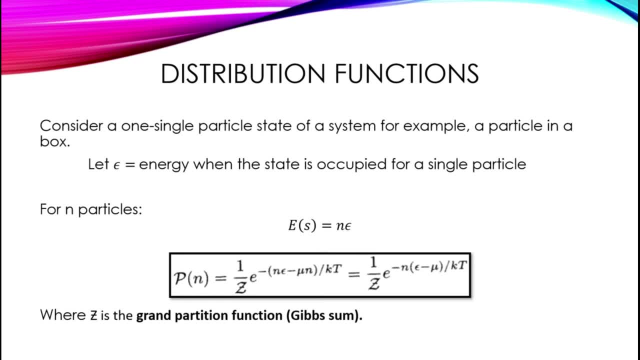 So if we consider this one single particle state as an example- a particle in a box- we can let epsilon be the energy When the state is occupied by a single particle. Then if we have n particles, the total energy of that system would be n epsilon. 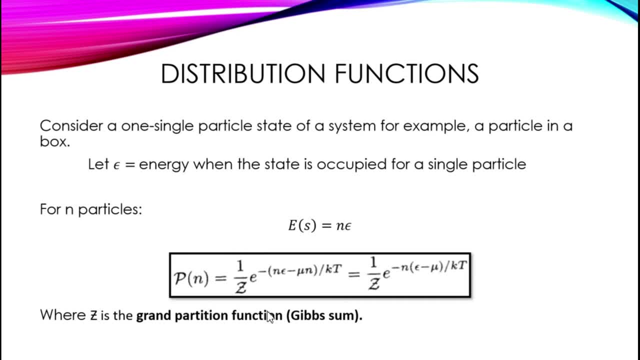 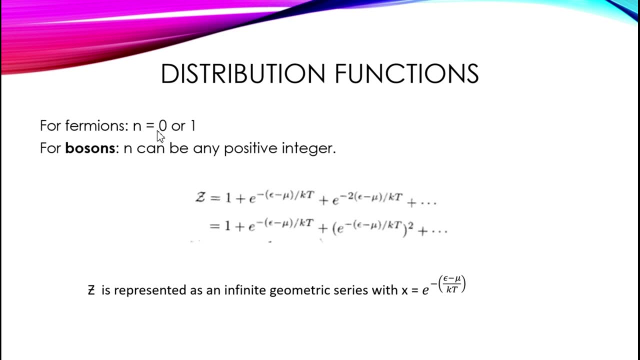 So then, the probability of the state being occupied by n particles is given by this equation, And again, z is the grand partition function, And recall that the sum of probabilities is 1.. So, for fermions, n is only 0 or 1,. 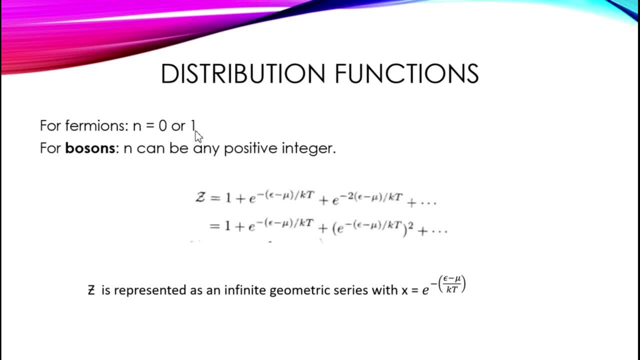 because only 0 or 1 particle can occupy the same state, But for bosons n can be any possible integer, So technically z would be an infinite sum. We can represent this sum as an infinite geometric series with x defined by this expression, the exponential part. 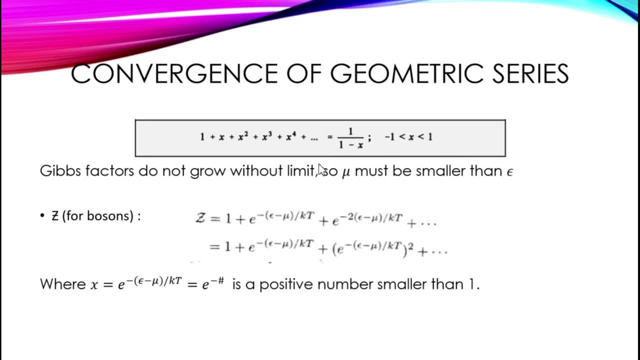 So then the convergence of geometric series tells us that if x is between negative 1 and 1, then this sum converges. So in this case we know that Gibbs factors do not grow without limits. So mu must be smaller than epsilon. 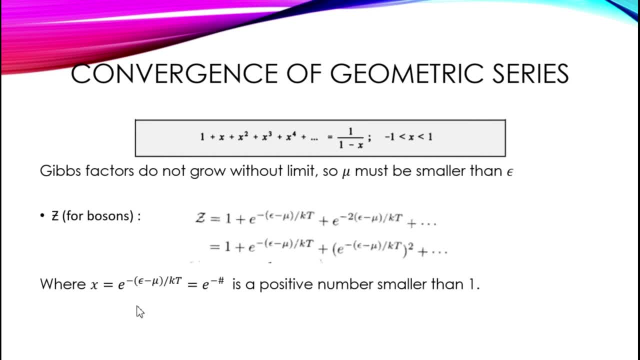 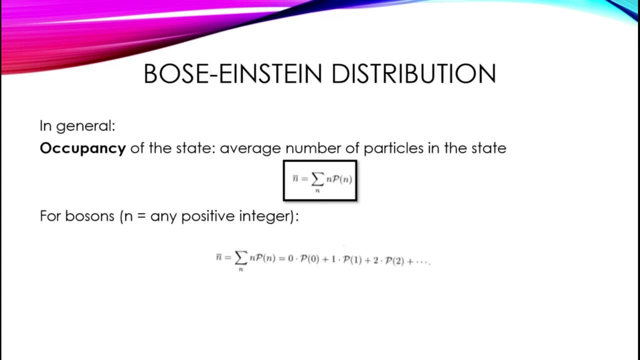 which means that the exponent part, like our x, is e to the negative number and it's a positive number smaller than 1. So this geometric series does converge. So for bosons it converges to this expression here. So if we want a more general description, 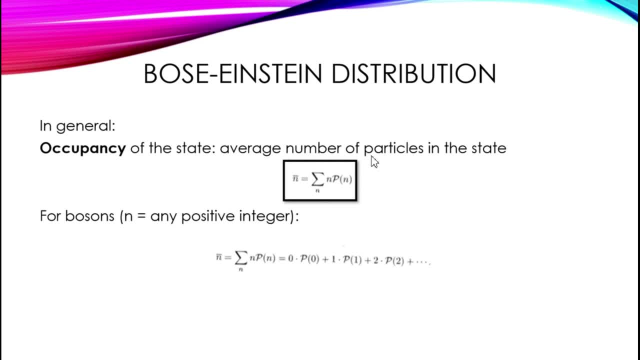 the occupancy of the state is defined as the average number of particles in the state. So n is n with a part on top. So for bosons, remember that n is any possible integer, So this is also an infinite sum. Now recall our substitutions from before for x. 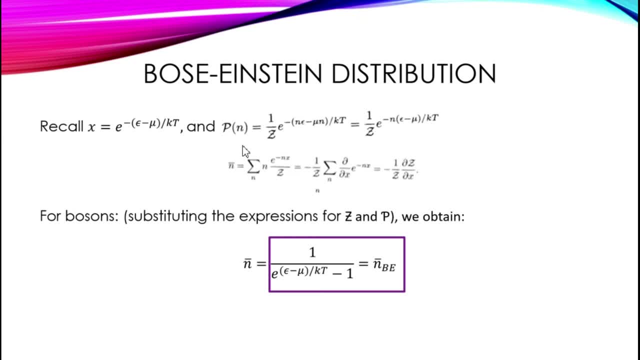 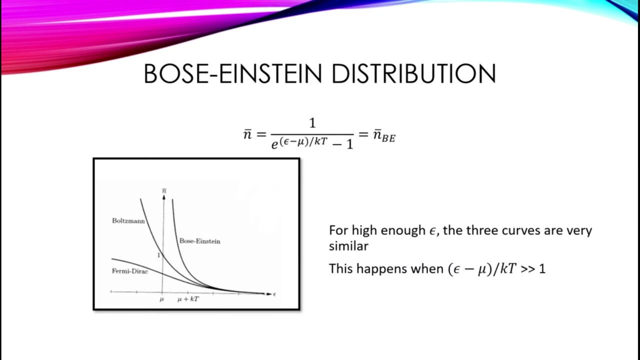 and the probability equation that we found before. So plugging this in in our expression for occupancy, we get this expression and then we obtain this from replacing our x and our p, And this function is the Bose-Einstein distribution. So here at the end. 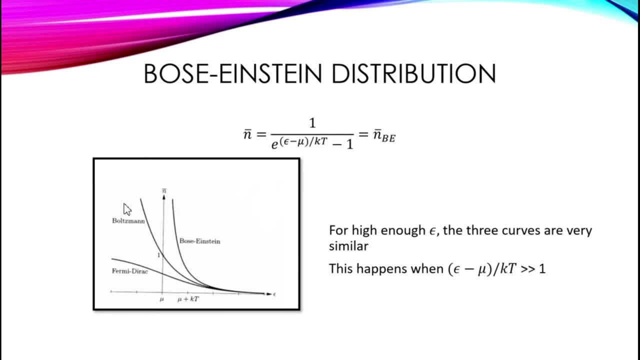 you can see a graph of the Bose-Einstein distribution, the Boltzmann and the Fermi-Dirac. For Fermi-Dirac, Fermion's n is just 0 or 1.. For the Boltzmann, there's no particle transfer. 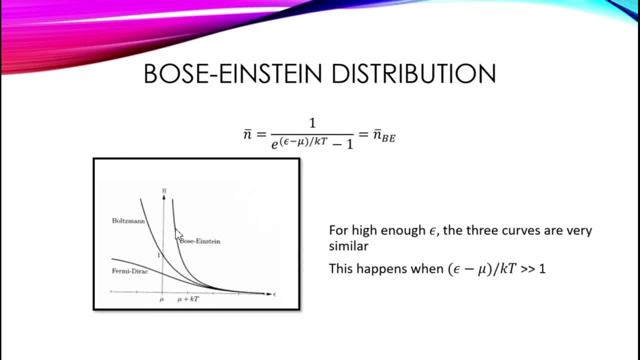 which we saw in chapter 6.. And for the Bose-Einstein distribution, it's about bosons and there is particle transfer and it can be any positive integer. Now look at this region here For a high enough epsilon energy of a single particle. 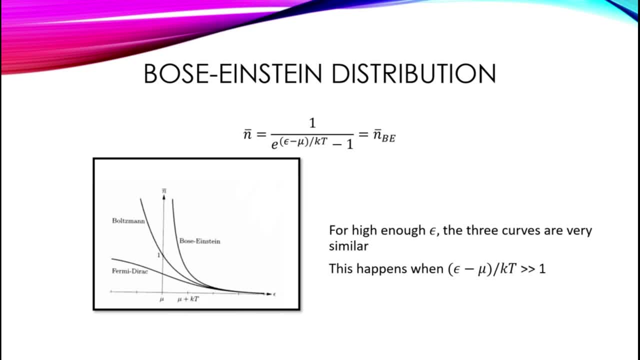 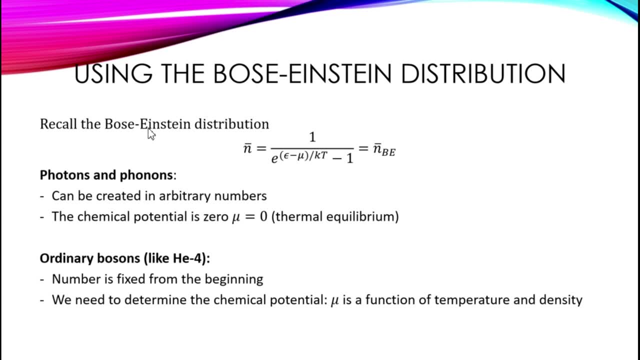 the three curves are very similar. So how do we use this Bose-Einstein distribution? So recall the Bose-Einstein distribution For photons and phonons we can just set the chemical potential to 0 and assume thermal equilibrium. But for ordinary bosons like helium-4,. 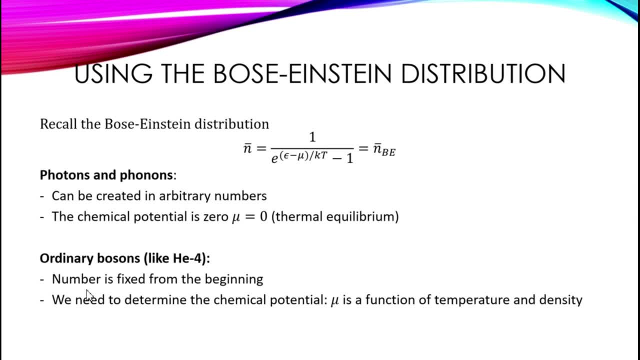 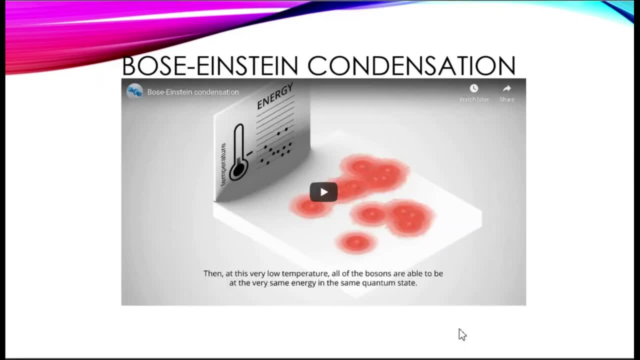 there is a number of particles already from the beginning, and we need to determine the chemical potential, which is a function of temperature and density. Now that we have learned the mathematical tools that we need to describe Bose-Einstein condensation, let's take a look again at what it is we're trying to describe. 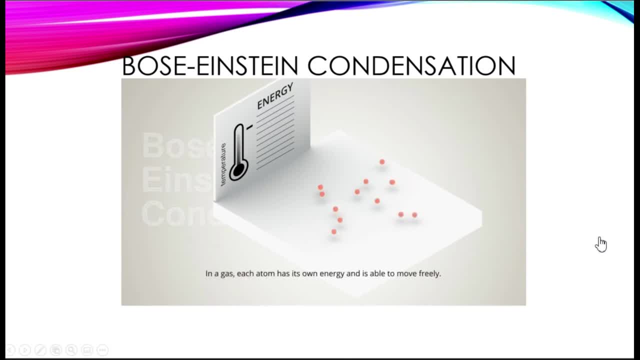 So let's go over to the last image and we'll have a look at the time difference And we'll take a look at the time difference. So this is the time difference between the two. So we'll start by taking a look at the time difference. 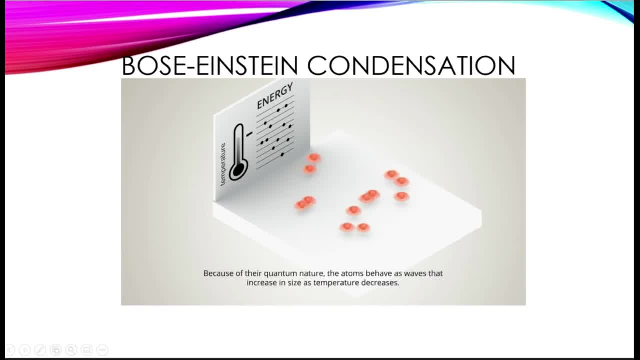 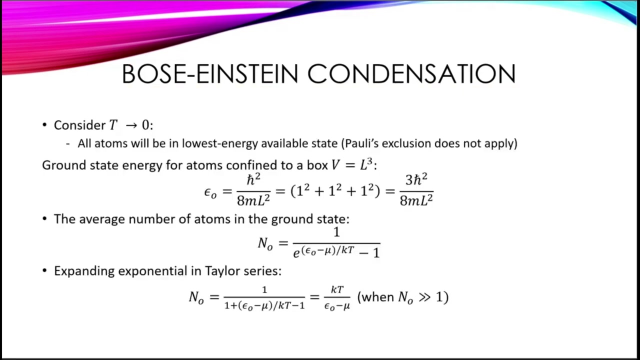 between the two, And what it means is that the time difference between the two is equal in the mass of the particle, which is 0.. Thank you, And now we can describe what we just saw. So consider temperature as it goes to zero. 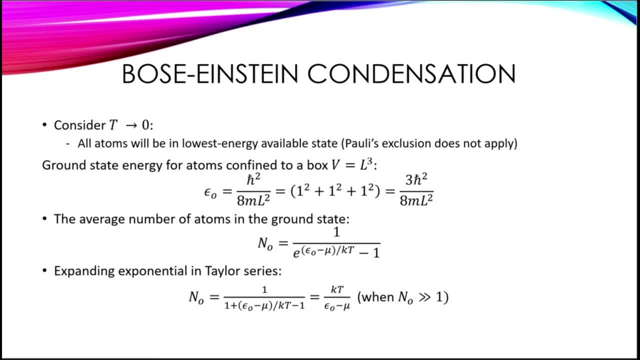 All the atoms will be in the lowest energy state available, because Pauli's exclusion principle does not apply. So if we consider the ground state energy for atoms confined to a box of volume, L cubed, then the energy in the ground state of a single atom can be defined by the equation given. 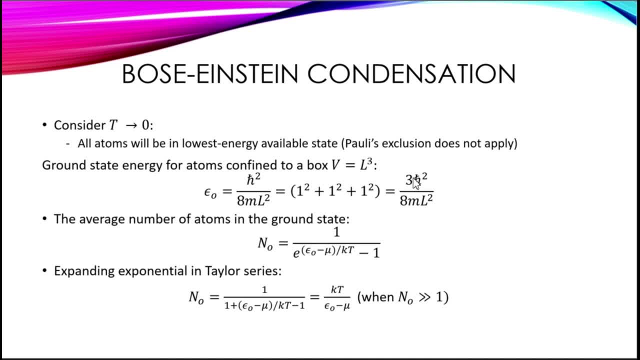 So then we can compute the average number of atoms using Bose-Einstein distribution. We're interested in the atoms in ground state, so we will call this N-naught, So that is given by the Bose-Einstein distribution, And then if T is low enough, N-naught is large, because many atoms will be in the low energy state, right. 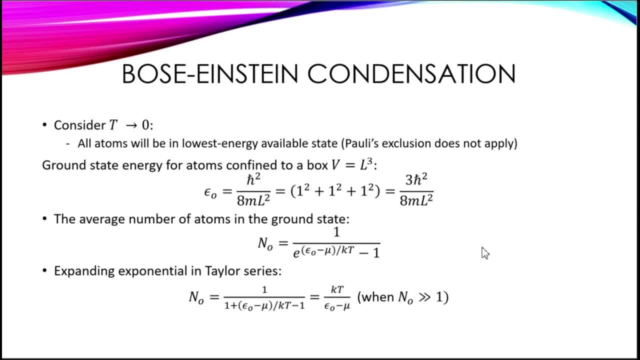 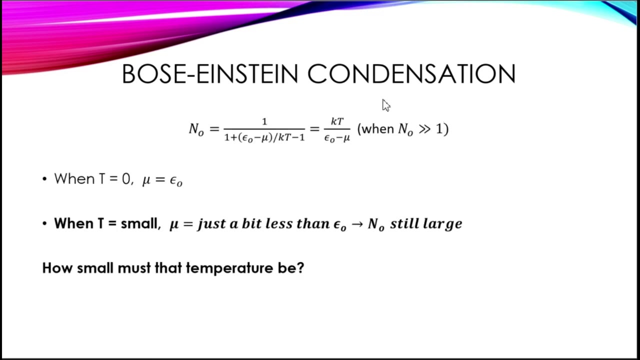 And this? We know this because the denominator must be small, right, The exponent is small, as T is low enough, And then the exponential part can be expressed as a Taylor series, and we can consider only the first two terms. So we get this. 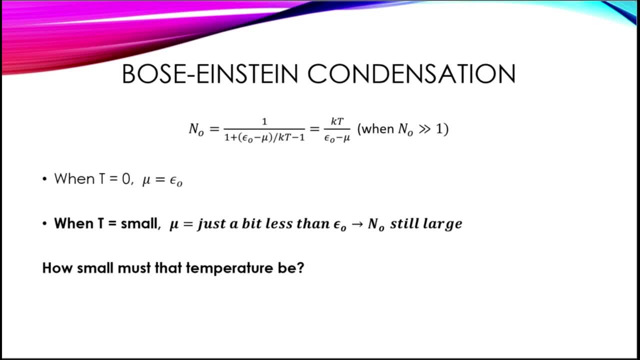 And when T is equal to zero, the chemical potential has to be equal to the of ground state energy of an atom. But when T is not zero, but it's small, mu is just a little bit less than E-naught, so N-naught is still large. 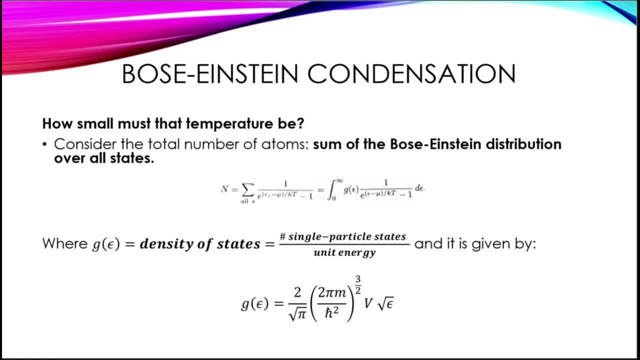 So how small must that temperature be? So to answer this question we need to first consider the total number of atoms, which is the sum of Bose-Einstein distribution over all states. Here we can convert it to an integral over the individual N-naught. 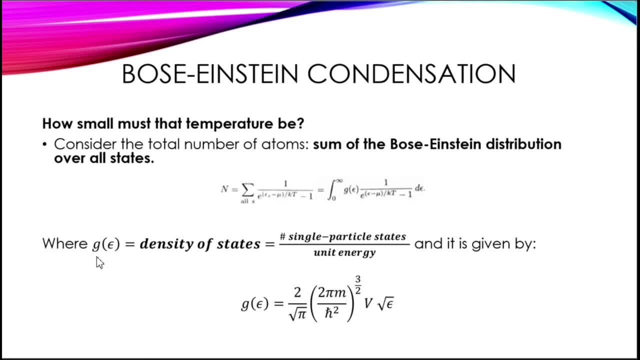 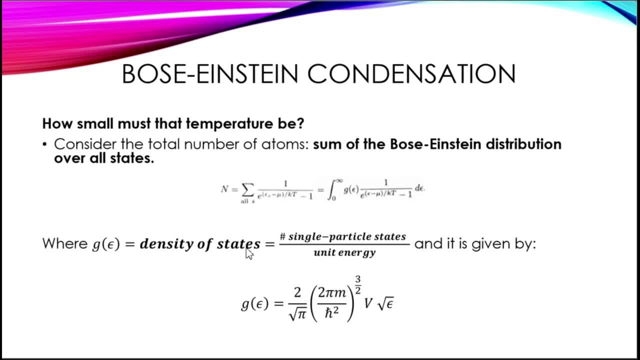 So G, e, G. epsilon is the density of states, which is defined as the number of single particle states over unit energy, And it is given by the following equation: where V is the volume, H bar is Planck's constant divided by two pi. 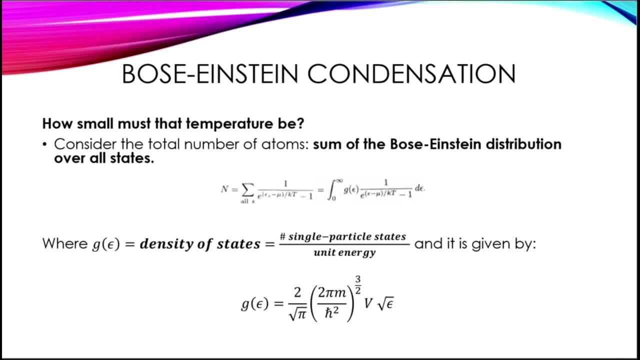 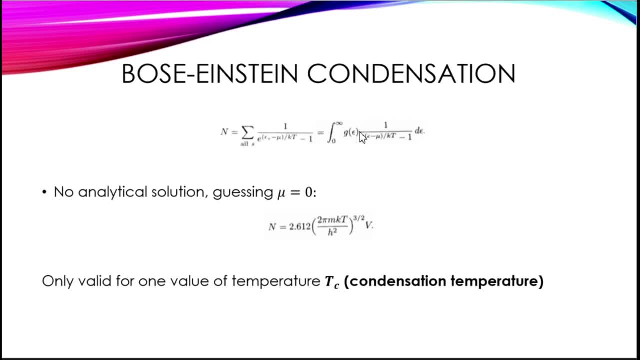 epsilon, the energy of a single atom. So this integral unfortunately does not have an energy, not have an analytical solution, and we must guess the value of mu. I started with a guess of mu equals zero. That gives us this expression, But this expression implies that the number 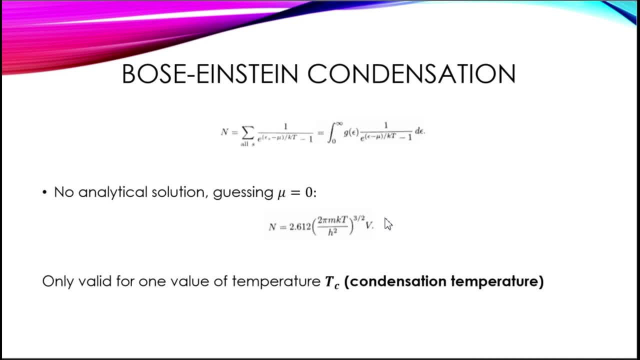 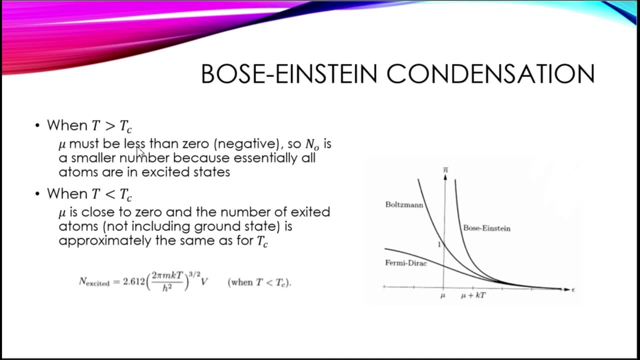 of atoms depends on temperature, which is not true. The answer is only valid for one value of temperature, which is the condensation temperature. So what happens when the temperature is greater than the condensation temperature? Well, mu must be less than zero, It should. 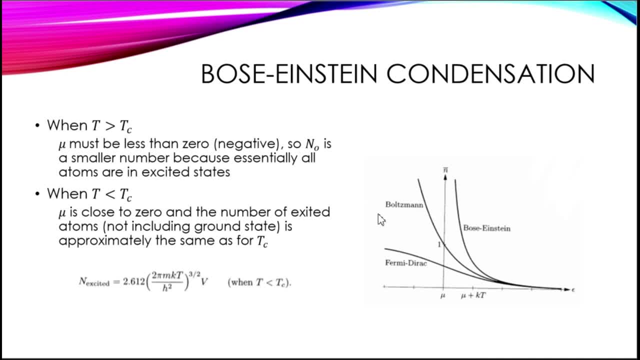 be negative, so that n0 is a smaller number, because essentially all the atoms are in excited states. So remember, n0 is the number of atoms in the ground state When the temperature is lower than the condensation temperature, mu is close to zero and the number of excited 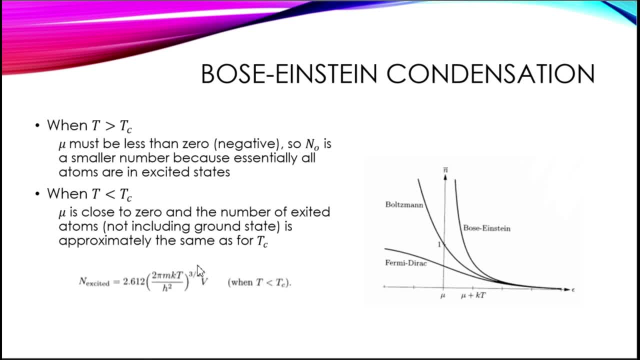 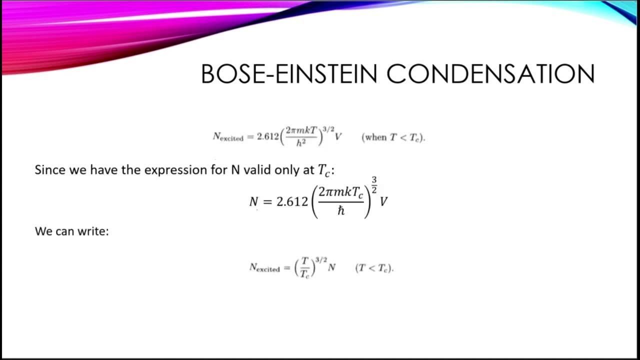 atoms, not including ground state, is approximately the same, But in this case the expression on the right-hand side looks the same, but n is not n0, it is n excited. So we know the expression for n valid at Tz. 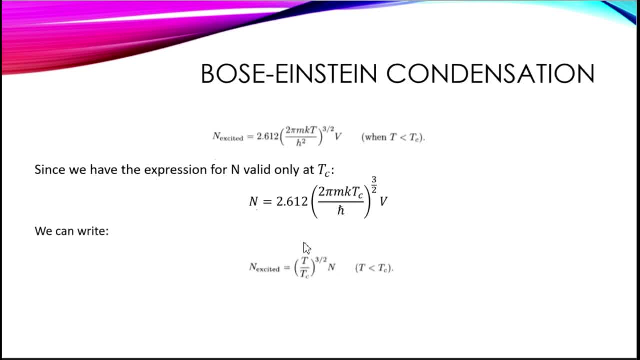 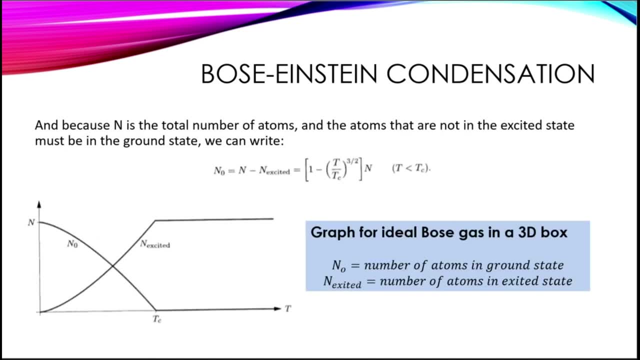 So we can write then the number of excited atoms as follows, And remember that the number of excited atoms is equal to the number of atoms in the ground state. So we can write then the number of excited atoms as follows, And remember that the total number of atoms is the sum of ground state atoms plus excited state atoms. So we 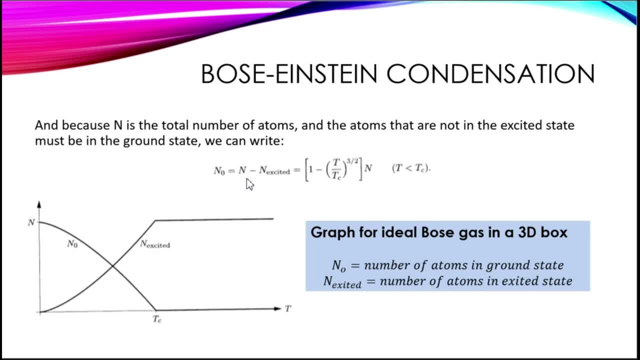 can write the number of ground state atoms as the total atoms minus the excited atoms And we get this expression. Now, if we graph this- the number of atoms in ground state versus temperature and the number of excited atoms versus temperature- we can see that 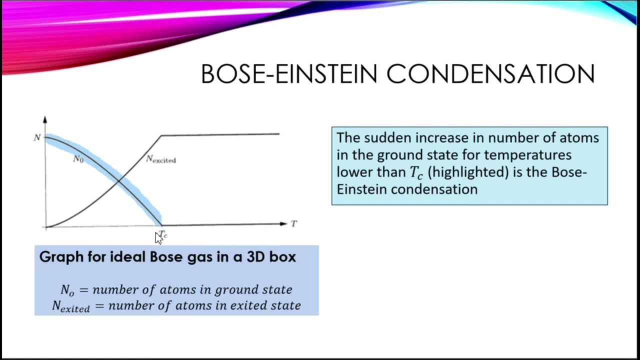 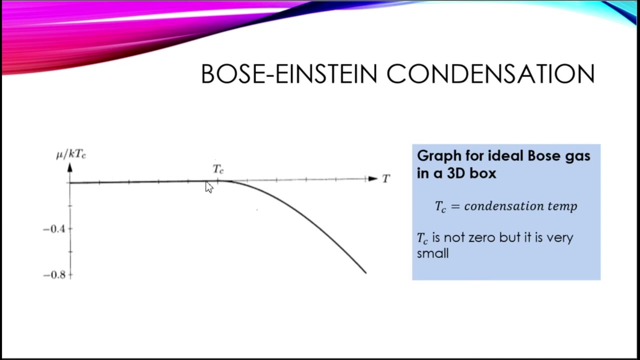 there is this sudden increase. as we go lower In temperature, we go below the condensation temperature. there is an increase in the atoms in the ground state. So that is the Bose-Einstein condensation And we call those atoms that appear here the condensate. We can also look at a graph of temperature dependence on the 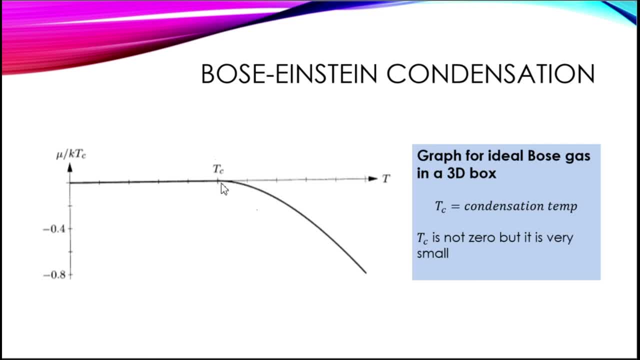 chemical potential. We can see here: Tz looks zero but in reality it is zero. So we can see that it is very small and the temperature is the initial drop on the temperature in the ground state. Now let's talk about the evidence for Bose-Einstein condensation. So Einstein's predictions were: 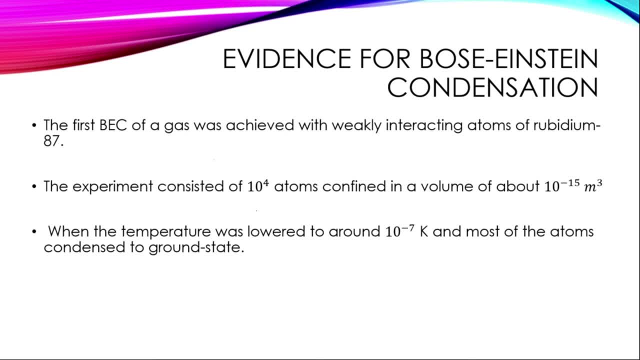 not verified experimentally until 1995.. The first case was a gas achieved with weakly interacting atoms of rubidium-87. This experiment consisted of 10 to the 4 atoms confined in a volume of about 10 to the negative 15 meters cubed. When the temperature lowered, the Rubidium-87 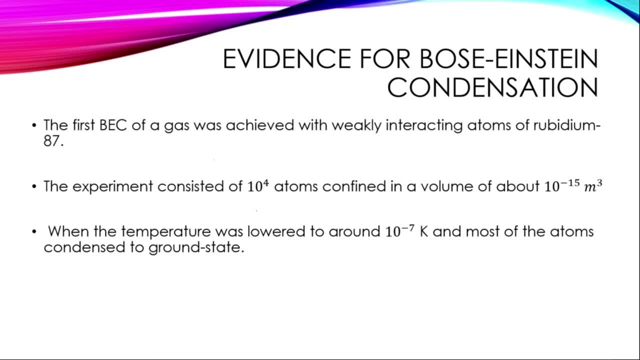 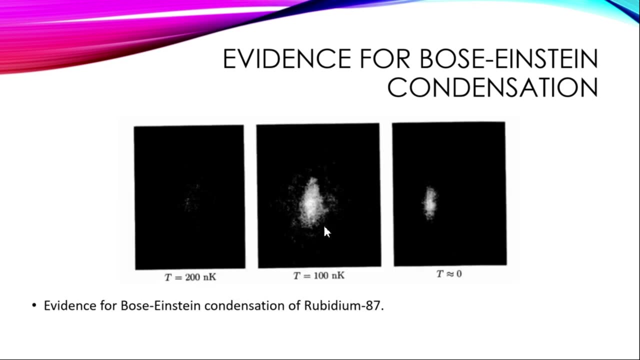 was released to around 10 to negative 7 Kelvin. most of the atoms were condensed to ground state. This was surprising because the individual atoms would normally be in the ground state at temperature a hundred times lower than that. Here we can see the pictures of that experiment. So in the first 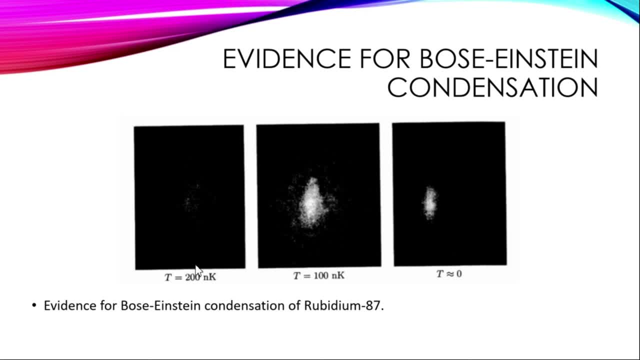 picture here above the condensation temperature. the velocity distribution is broad and isotropic and it's described as Maxwell-Boltzmann distribution. Below the condensation temperature, which is this middle picture, most atoms fall into a small region in the loss of space and the atoms. 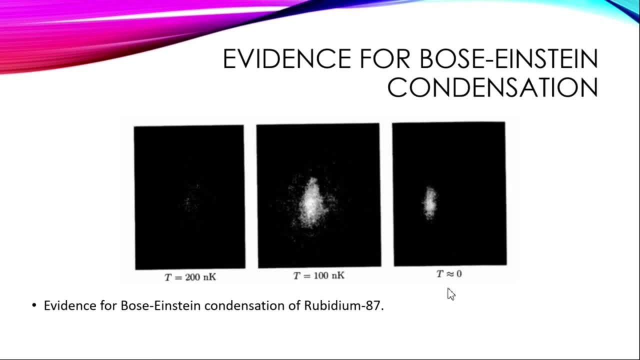 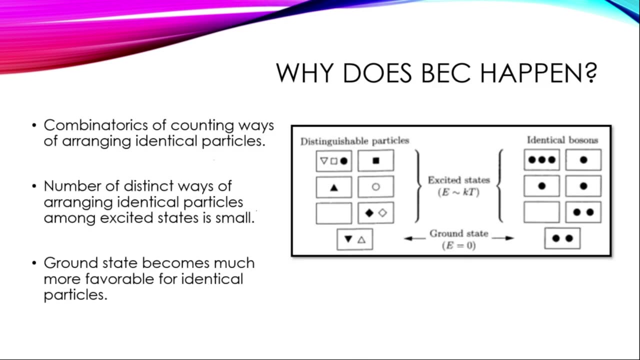 we're seeing here are the atoms that form the condensate, And at the temperature of approximately absolute zero. essentially, all the atoms are in the ground state wave function. So why the condensation? Why does Bose-Einstein condensation happen? Well, it happens because of the combinatorics of 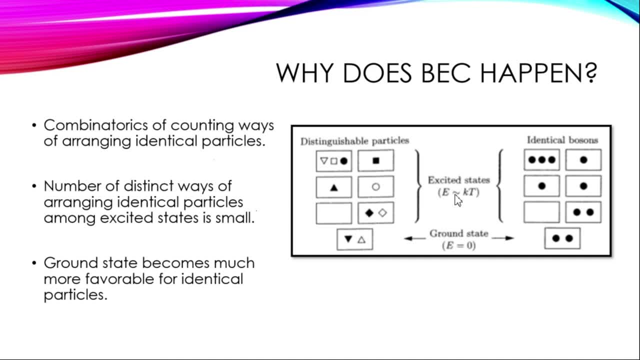 counting ways of arranging identical particles. As we can see in these graphs, the number of distinct ways of arranging identical particles among excited states is very small. compared to those of particles that are distinguishable, You can arrange them in many more different ways in excited states. So in the case of identical particles like bosons,